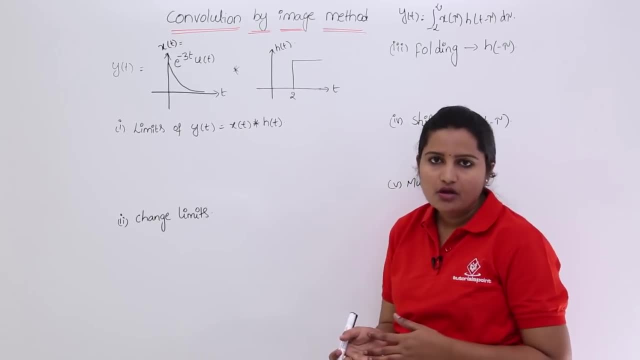 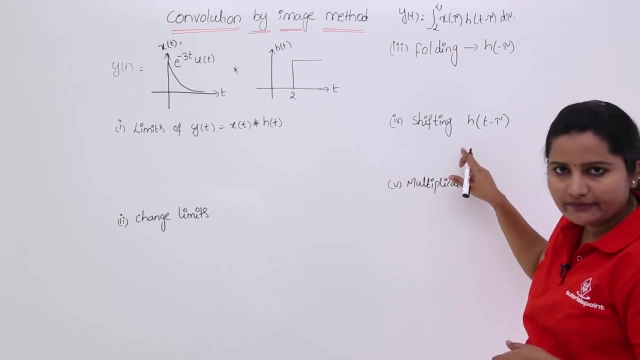 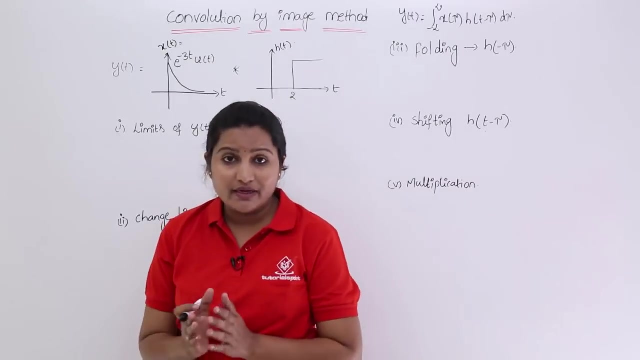 limits and change your time axis into tau after that. So you need to perform two actions about this: shifting and folding. first you need to fold and then shift. finally, multiplication of x of tau and h of t minus tau you need to perform- Now I am estimating the limits- 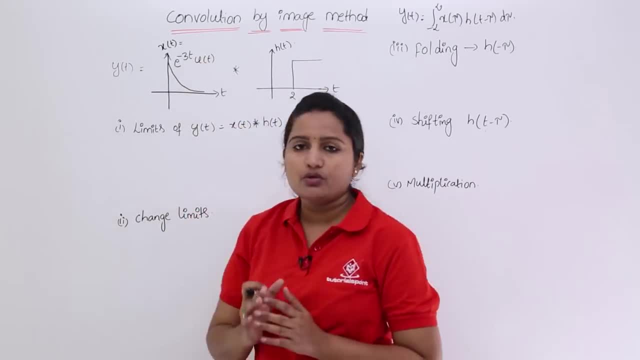 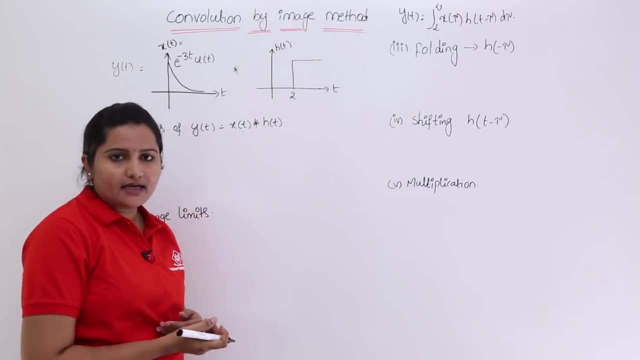 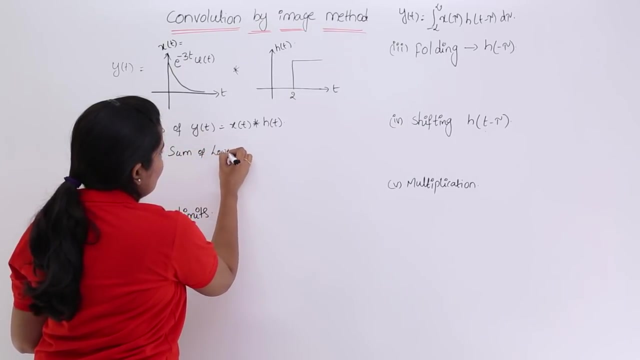 limits of your convoluted signal. so here we know the equation for estimating the limits of convoluted signal, that is: sum of lower limits less than t less than sum of upper limits. so here, sum of lower limits, lower limits less than t, less than sum of upper limits. 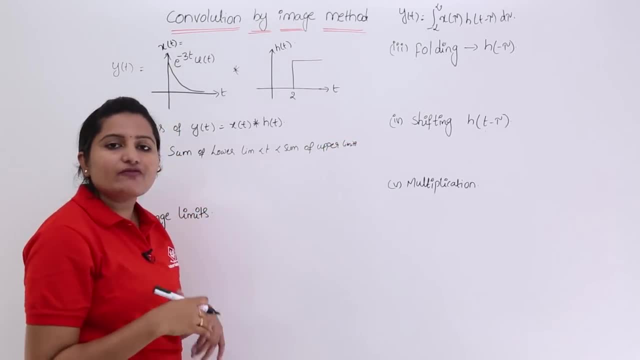 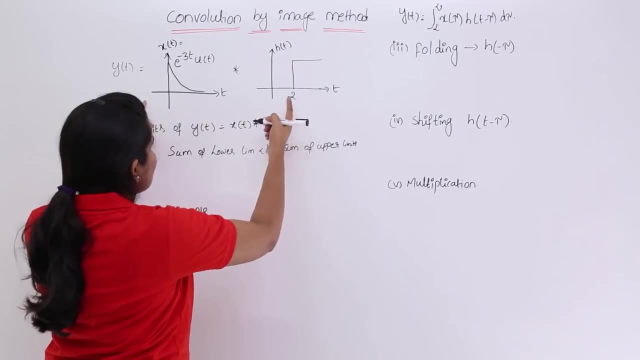 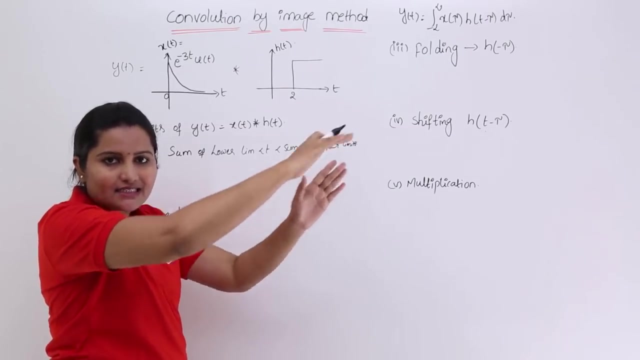 so this is the formula to estimate the limits of convoluted signal. so convoluted signal limits, or sum of lower limits of these two signals is. so here you are having 0. initially you know that e power minus 3 t u of t ends at infinity. so here this is somewhere ends. 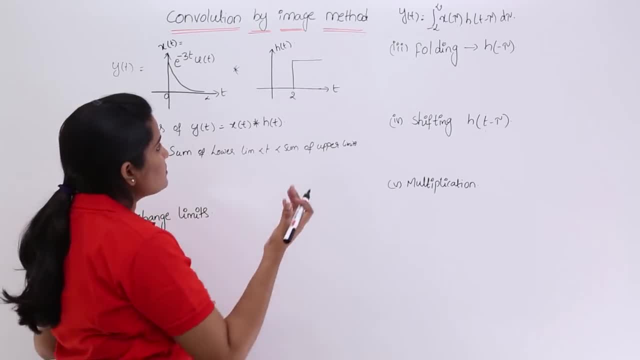 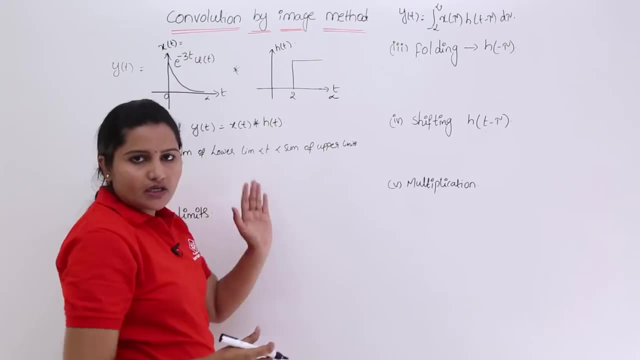 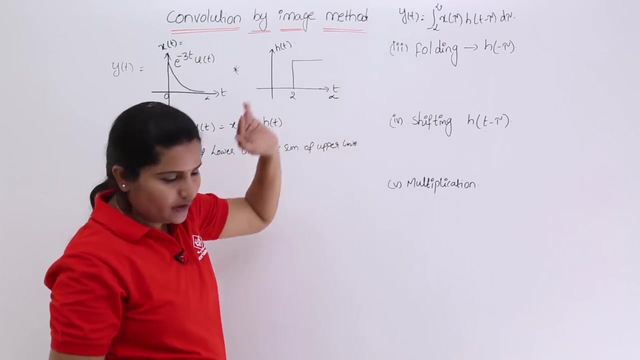 at infinity, that infinite at infinity, that value is equivalent to 0, but here so you are having 2 and here you are having 3.. So that means you are having t at infinity only. so that means it is a continuing signal up to infinity. this is also continuously, we are having signal up to infinity, at infinity. 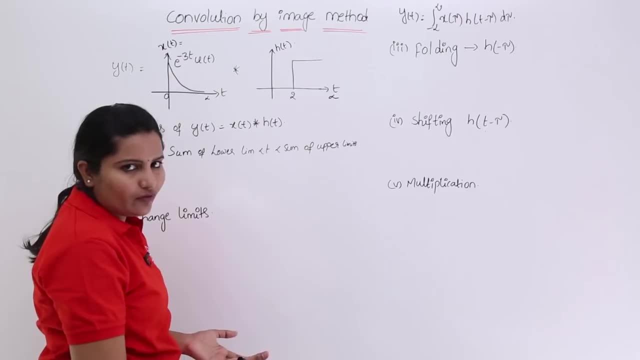 the value of signal is 0. but we don't want any value of the signal, we just want the limits: starting limit and ending limit. this signal is also not having any ending. this signal is also not having any ending because that is shifted unit step. Unit step is going to continue up to infinity, so this is also not having any ending. the 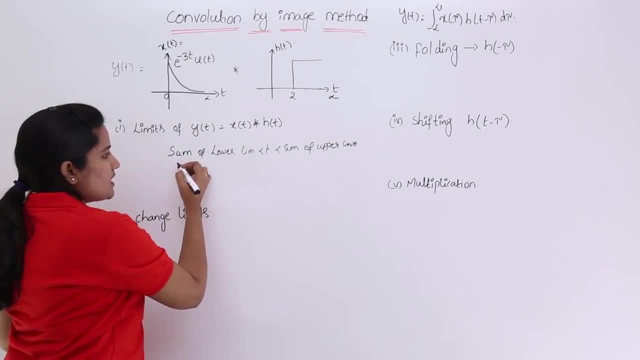 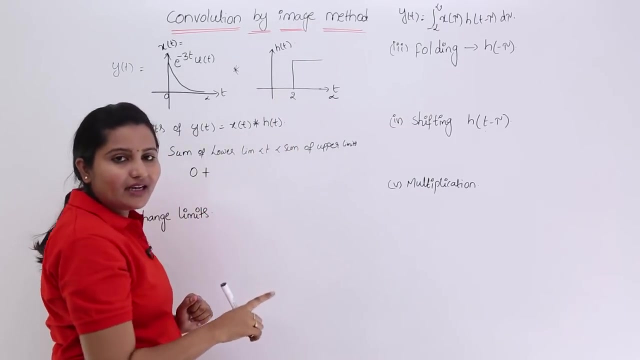 ending limit is infinity only, so here. so sum of lower limits means so here this is the lower limit of e power minus 3 t u of t signal, 0, plus. so here lower limit is 2. actually lower limit of unit step function is 0, but that is they given as shifted function, so shifted. 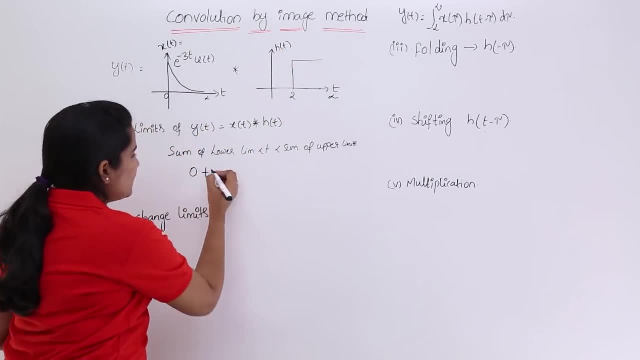 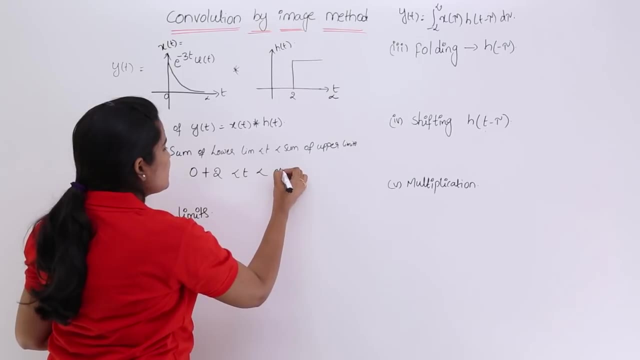 unit step they considered as impulse response here. So here that lower limit is 0. So here lower limit is 2. less than t, less than sum of upper limits is for both upper limits are infinity, so infinity plus infinity. so you are going to get 2 less than t less. 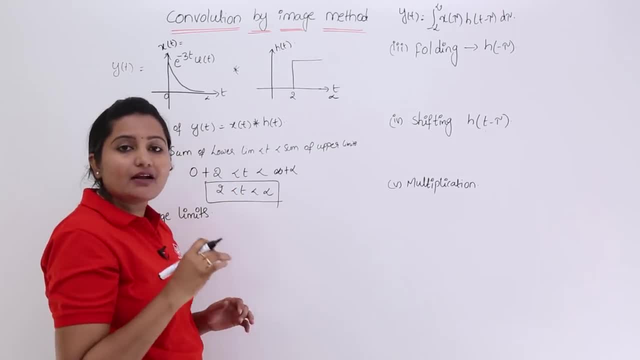 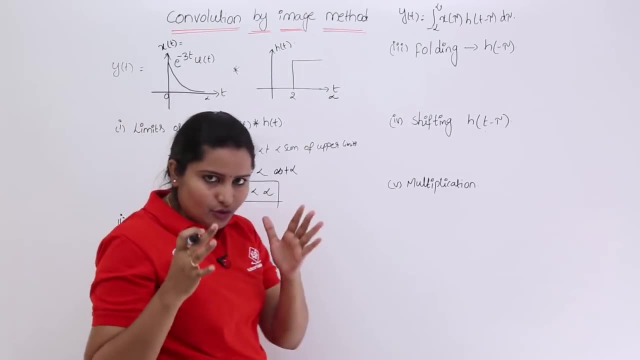 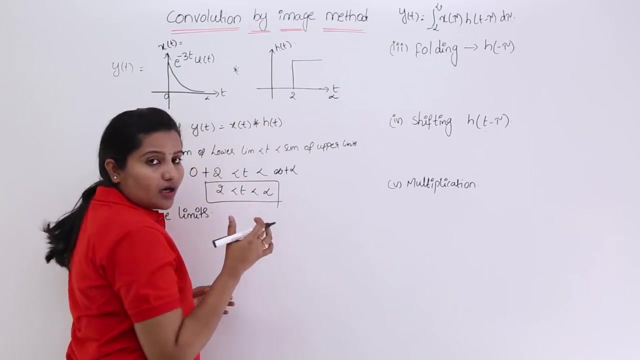 than infinity is your time limits for your convoluted signal. So your convoluted signal now having time limits from 2 to infinity, that means your convoluted signal is going to be present from 2 to infinity only. For example, if you are asked to find out the convolution, 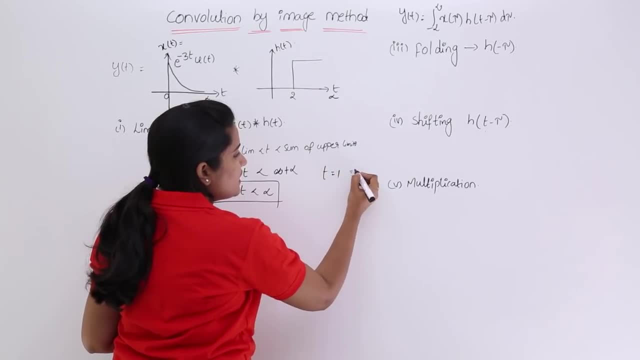 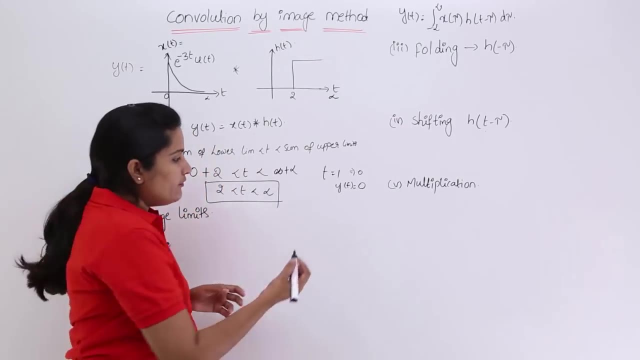 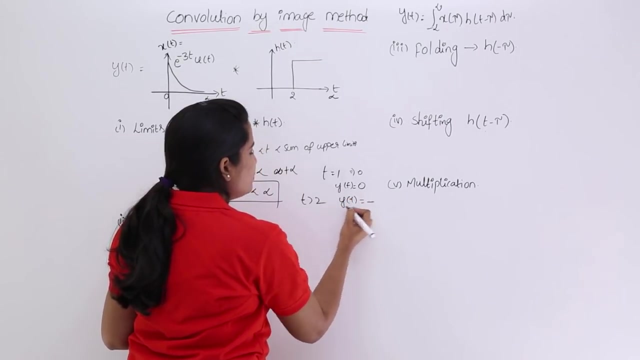 Limits. at t is equal to 1, means that is equivalent to 0. that means y of t is equivalent to 0. at t is equal to 1, that means greater than 2. when t greater than 2, you are having your convoluted signal. that means y of t is having some value. when t less than 2, your response: 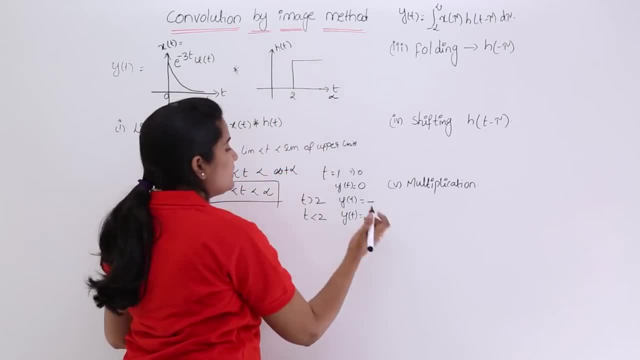 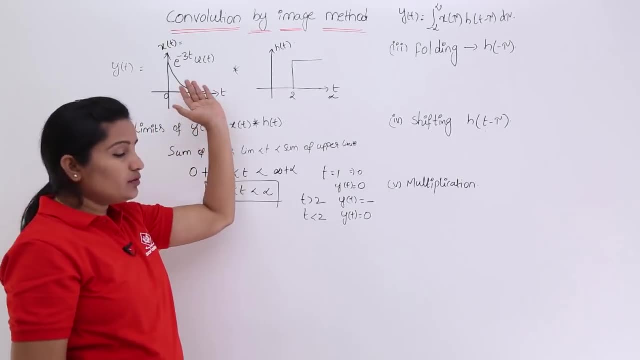 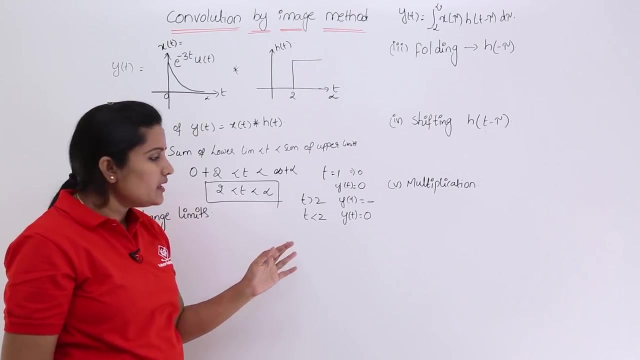 that means convolution of this signal and this signal is equivalent to 0.. So, for example, in any example, They can ask like this: they can give these two signals like this and they can ask: what is the convolution of your particular system at t is equivalent to 1 or 0, they may ask like: 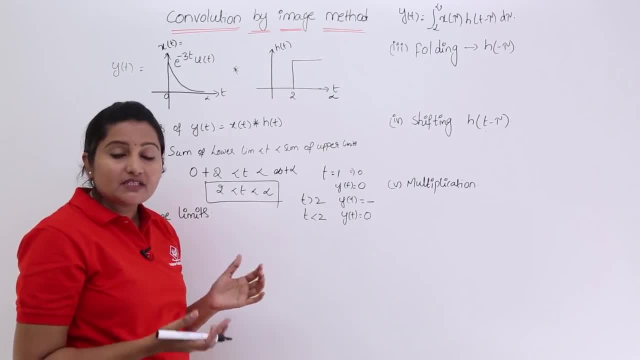 this at t is equivalent to 1 or 2. that means whenever t less than 2, your response of the system with convolution of these two signal will be is equivalent to 0. then you can say directly when they given t less than 2.. 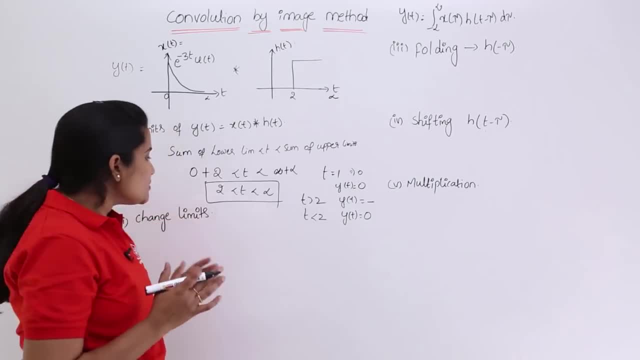 Then you need to Say: y of t is equivalent to 0. So now here: change the limits. so this is the next step that we need to perform: changing the limits. that means. so here we came to know our convoluted signal will be in this time. 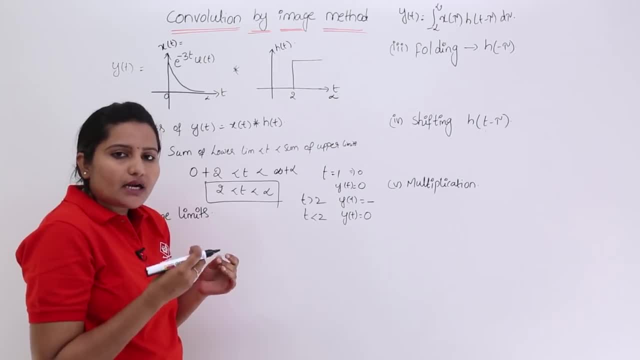 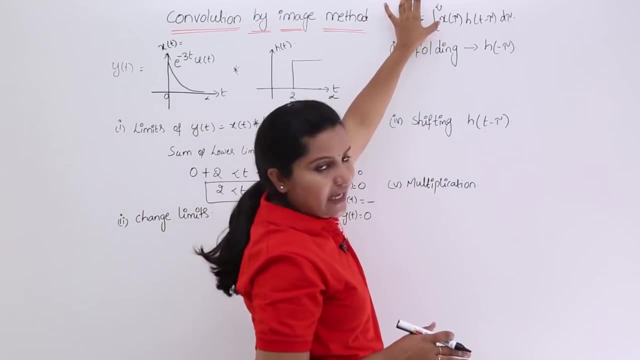 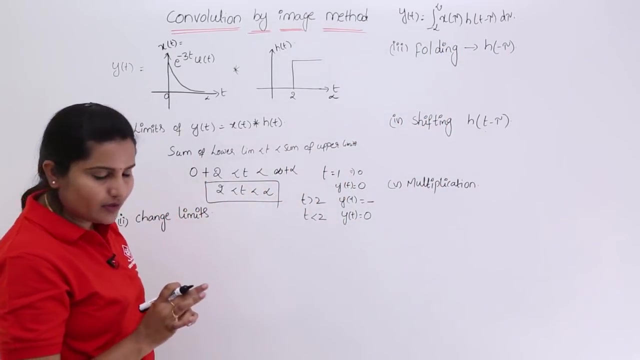 limits 2 to infinity. that is ok. So to cross check, at final we are going with this procedure now coming to here. So we are having this formula to calculate the convolution in that x of tau, h of tau, like that, are there. That means we need to change our time limits. 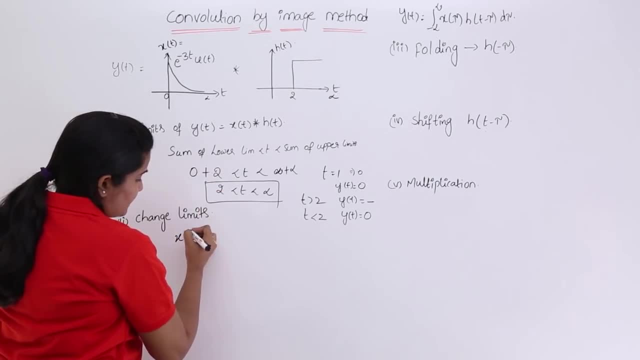 So here I am changing so x of t to x of tau. that means whatever signal I consider here, so that I am changing into tau domain. so changing the domain, that is it. So tau domain, that means c power minus 3 tau, u of tau. so here this is one thing and another. 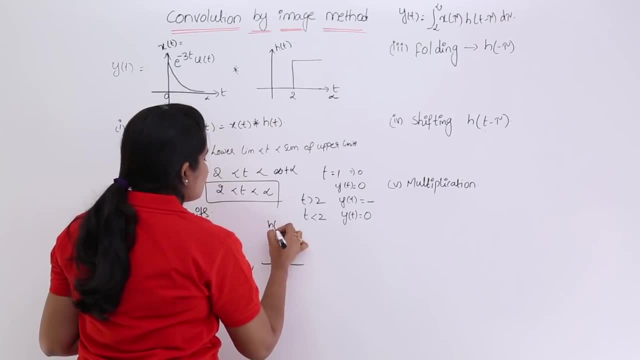 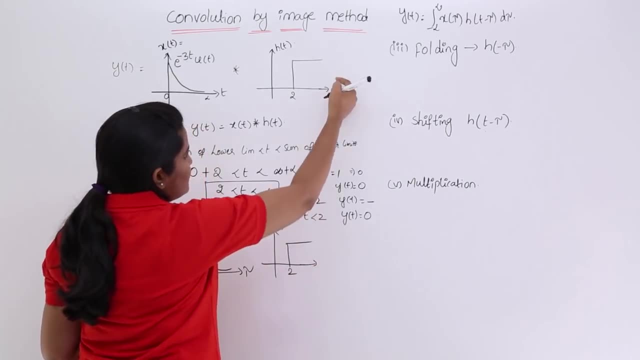 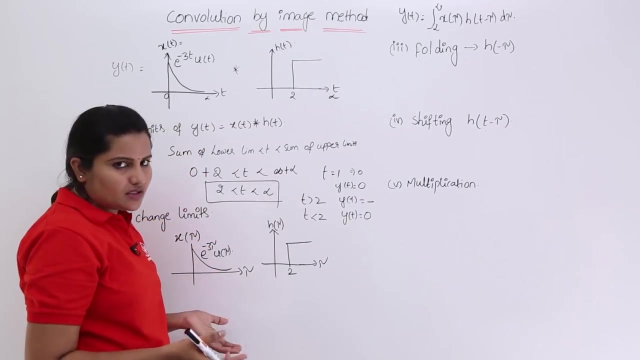 thing is h of tau. Ok, So this is h of tau. so actually we are having from 2 to infinity. So the x line is t here, but I am changing to tau. What we need to do is, in place of t, just substitute tau. 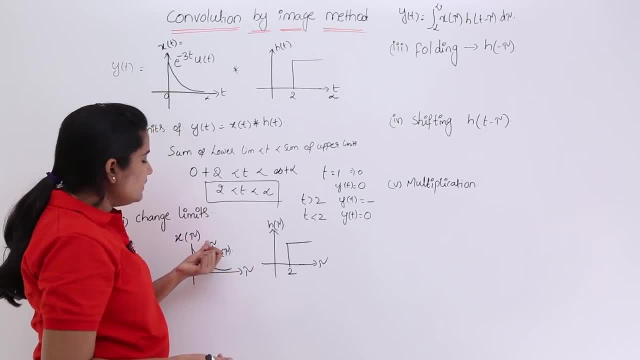 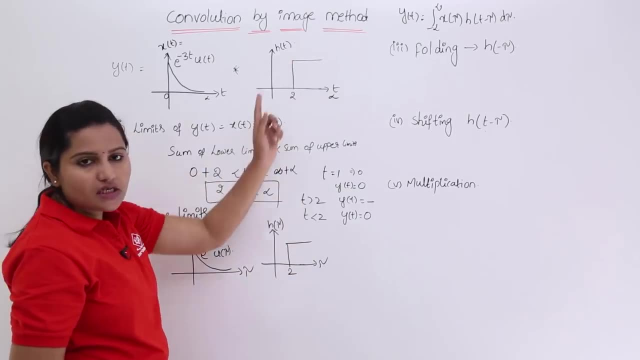 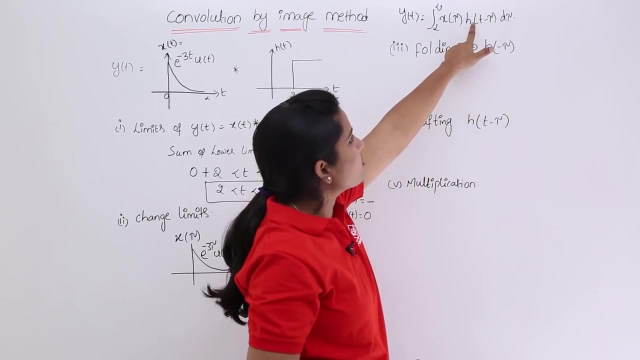 So x of tau tau. here. e power minus 3 t? u of t can be changed to: e power minus 3 tau? u of tau. So here also I am changing like that, So now. So here, after changing, we need to fold h of minus tau. why? because we need h of minus. 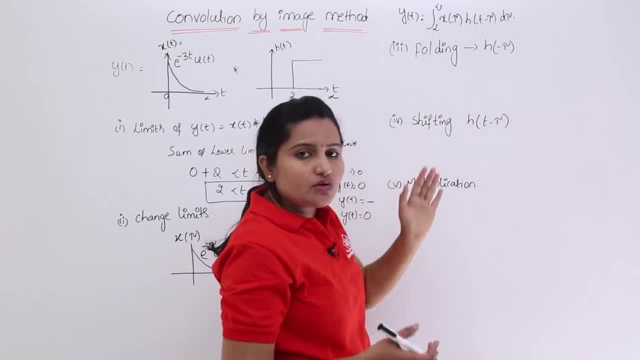 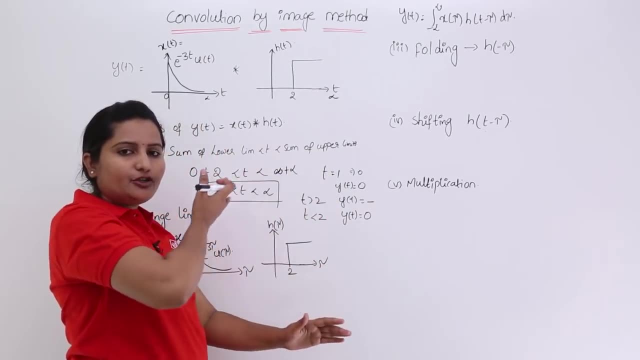 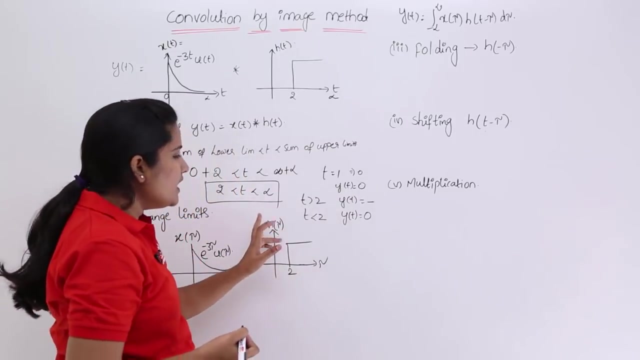 tau. that is also shifted h of minus tau. So shifting we will do later. first I am going to fold the signal. that means folding, or reflection, means we need to get the image format. So here, after folding, after getting h of minus tau, if this is h of tau, h of minus tau will. 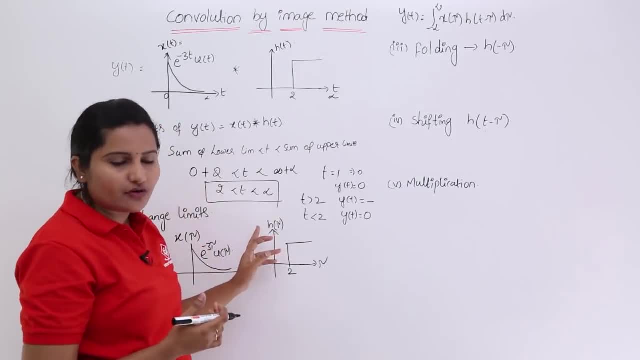 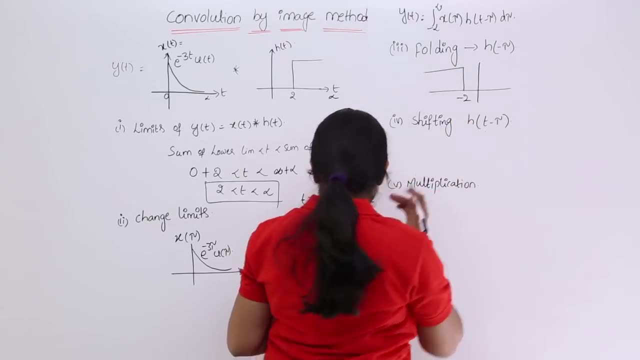 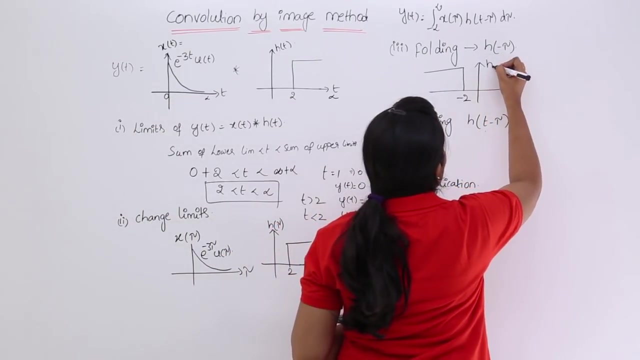 be the folded version or image version of h of tau. Ok, That means so you are going to get like this. so minus 2 from minus 2. here the signal is from plus 2. the image format will be like this: from minus 2. you are having your signal. 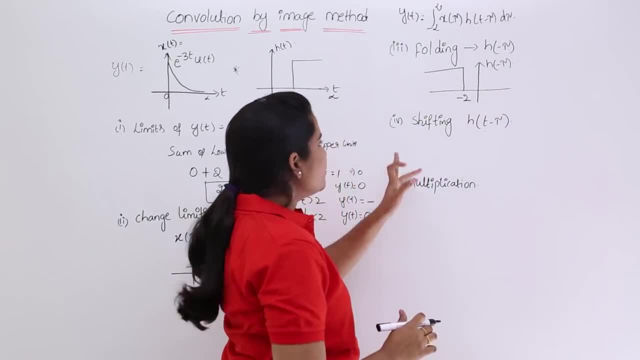 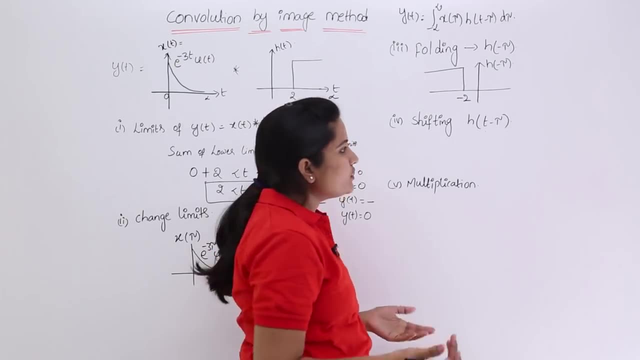 this is called as h of minus tau. So now you want your shifted version of signal. So how much shift it is undergone you do not know. So you need to have your shifted signal. This t may be either positive or negative. Ok, 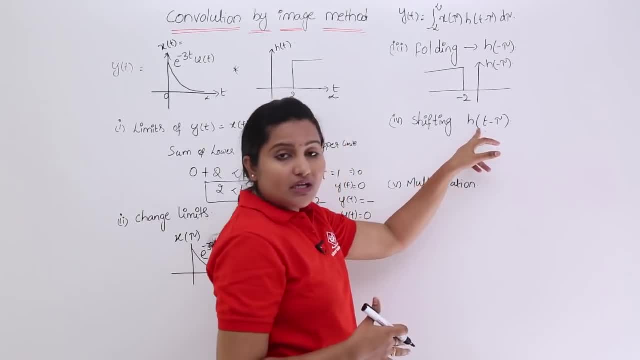 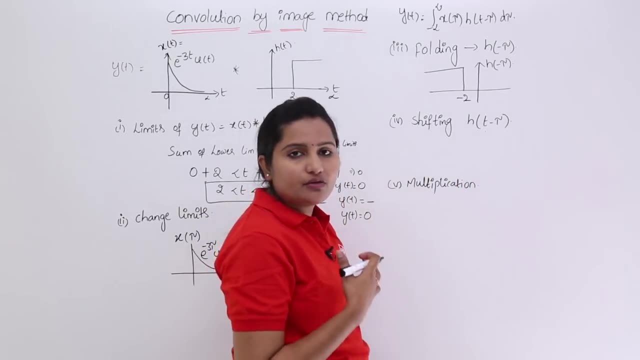 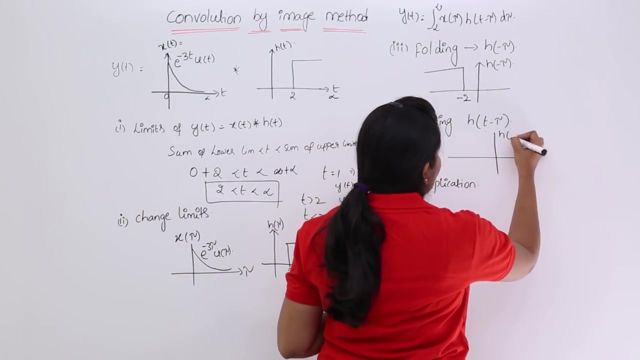 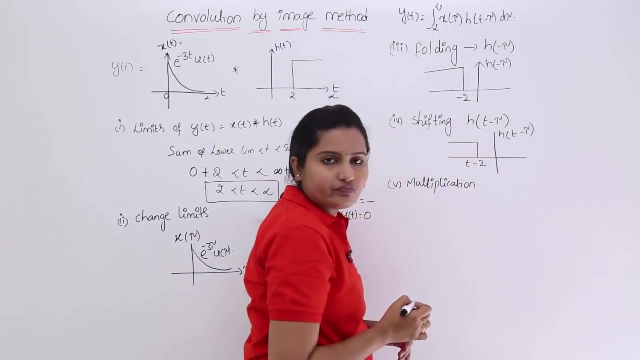 For example, if you consider this as positive, then you need to consider left shift. if you consider this as negative, then you need to undergo a right shift. So here, for example, I am considering like this: because of this shift, t minus tau. so you are going to get t minus 2 here. t minus 2 here. why? because if you consider t minus, 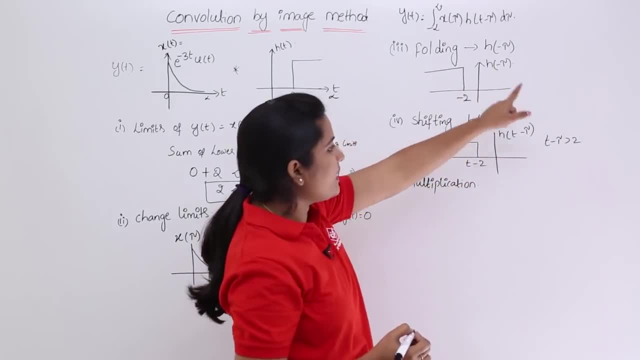 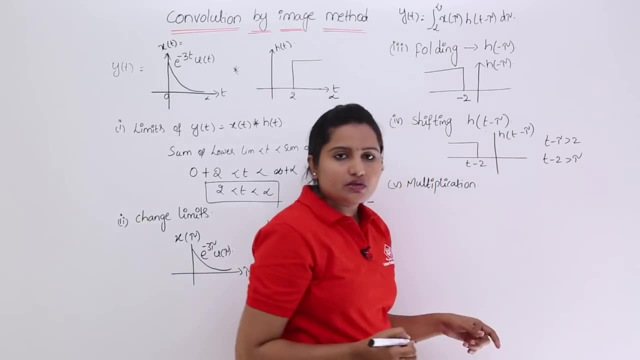 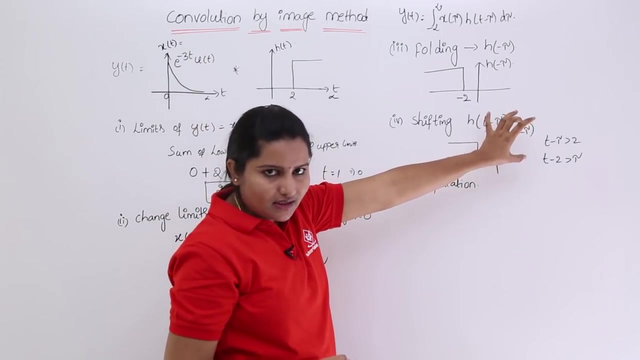 tau greater than 2. if you consider your t minus tau greater than 2, then you are going to get t minus 2 greater than tau. So that is why I am considering t minus 2 here. So like this your signal will be: by using this shifting, 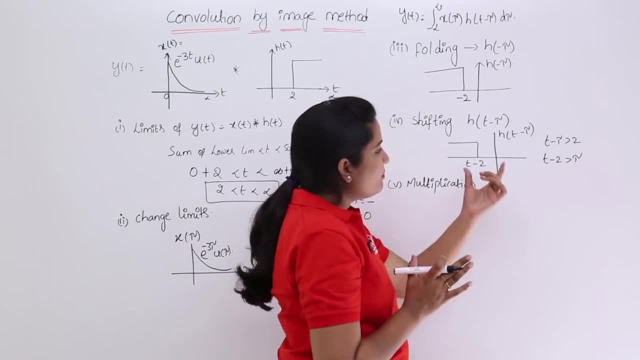 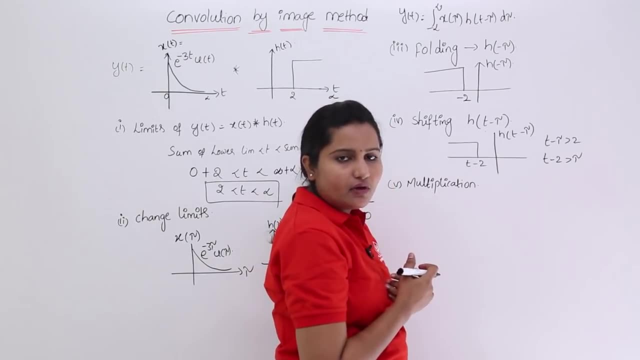 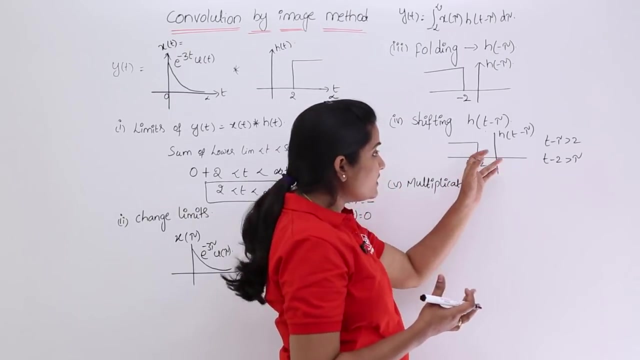 So after this I need to multiply. So before multiplying, I want to discuss with you something. for example, t greater than 0 or t minus 2.. Ok, So t minus 2. whatever t minus 2 value is there, if that is greater than 0, where this signal? 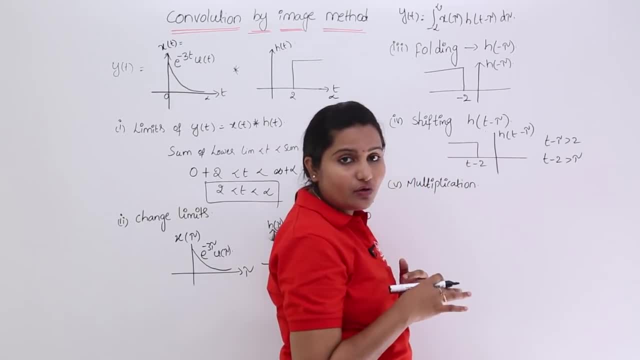 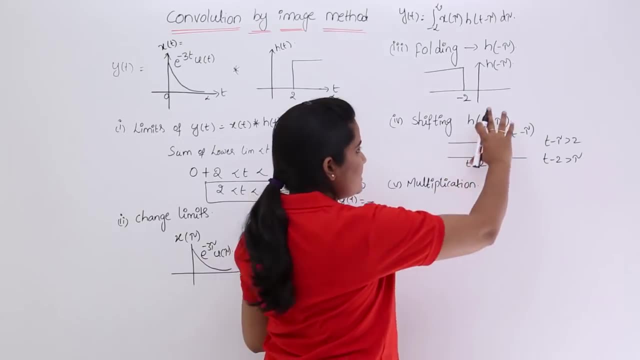 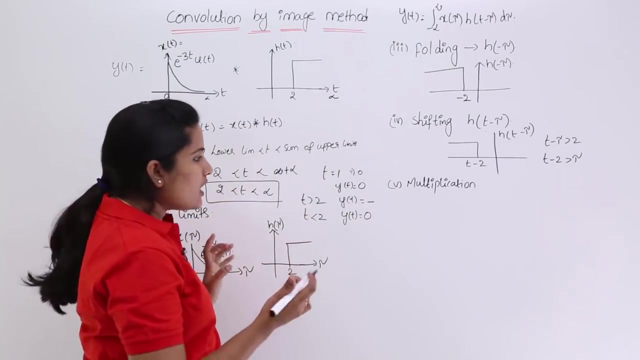 will present when t minus 2 is less than 0, where this signal will present. I will want to discuss with you, For example, in case of multiplication, this is h of t minus 2 signal and we are having h of tau signal like this: 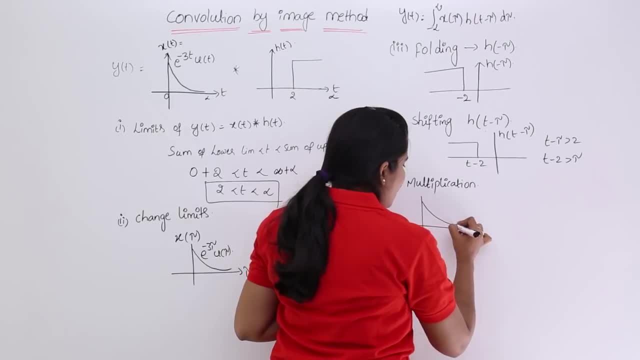 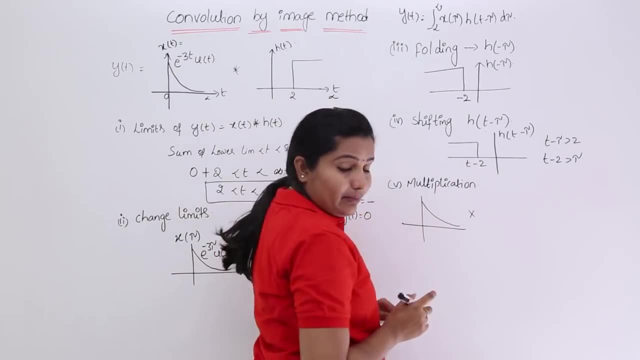 So I am just writing my h of tau signal and I am going to multiply. So if I want to multiply with this t minus 2, so if I want to multiply with the t minus 2, before getting into the multiplication I want to check whether the signal is going. 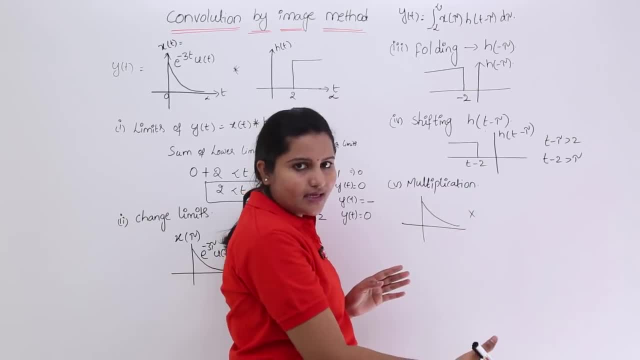 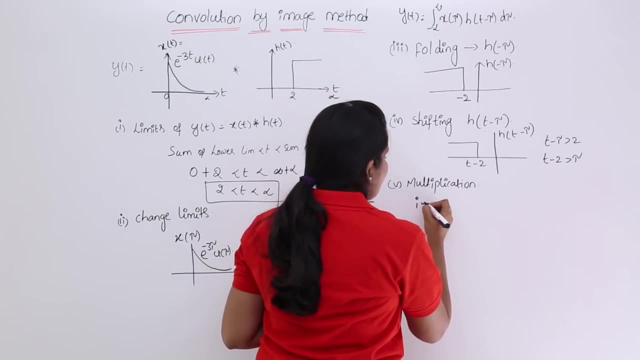 to present in positive x axis or negative x axis. So here, if I am searching one case: so if t minus 2 is greater than 0, that means if t minus 2 results greater than 0.. Ok, That means if t is a bigger value than 2, then what will happens? then this signal is starting. 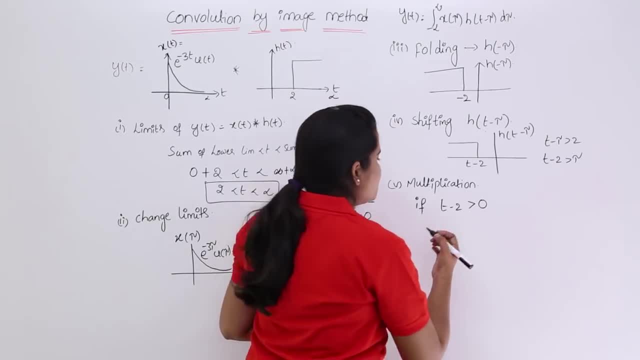 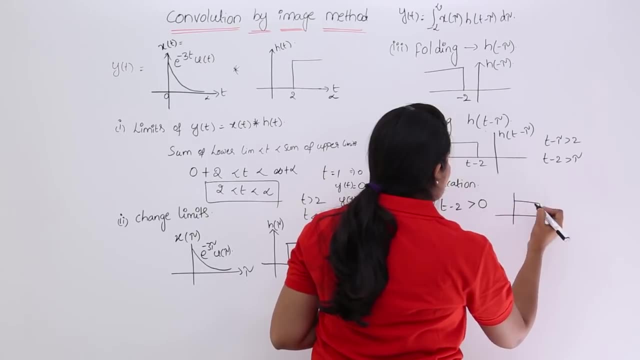 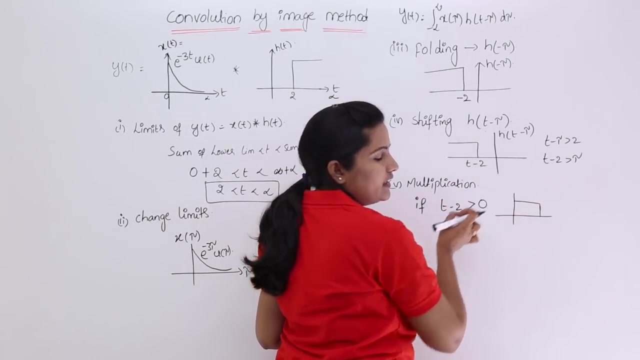 from, so 0 onwards. So that means so you are going to get so like this. so here you are going to get like this. so t minus 2 greater than 0 means you are going to get this value at anywhere here. So here and another signal you are having. 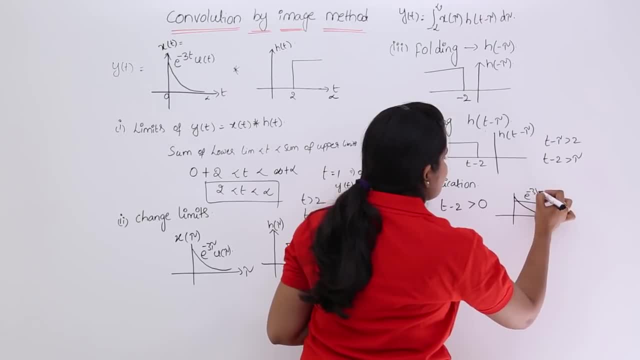 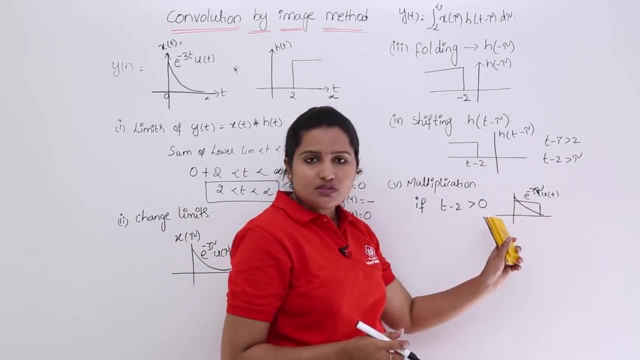 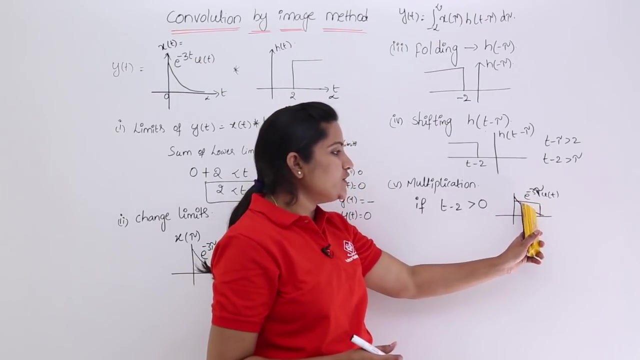 So you are having is like this: e power minus 3 t u of t, or e power minus 3 tau u of t, So multiplication of these two signals will takes place. in this case, multiplication of these two signals will takes place. that means so 1 into anything you are going to get. so 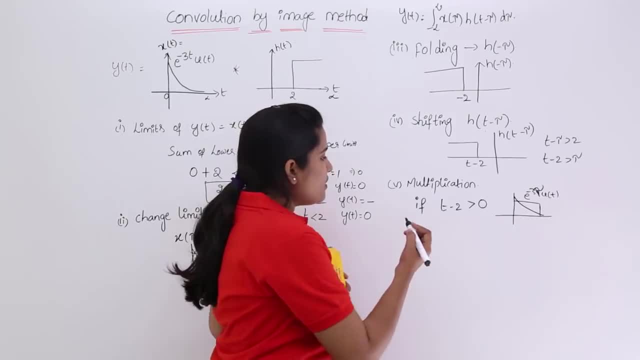 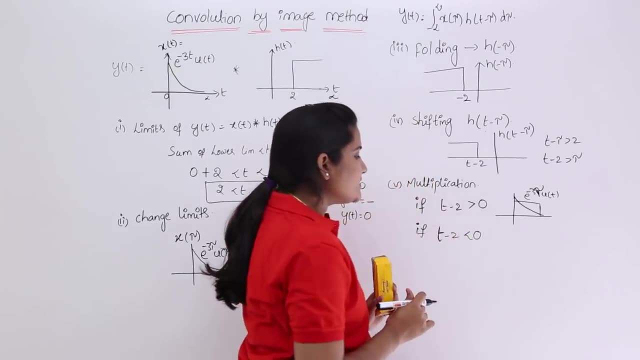 that e power minus 3 tau u of t only. So now, so if t, t minus 2 less than 0. Ok, So this is what we are going to get. Ok, So if t minus 2 is greater than 0, for example, if your limit, this limit, is less than 0, then 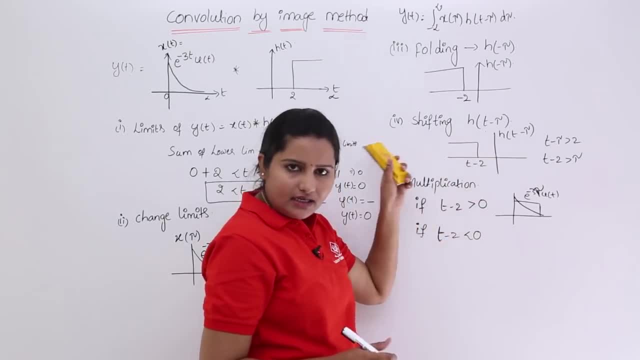 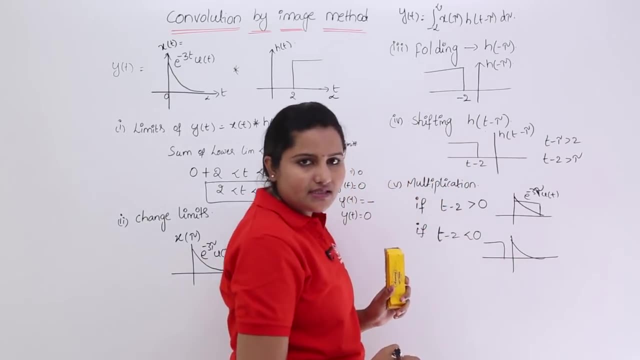 this signal will keep as it is, like this, in negative x axis, then what will happen when you are multiplying? your signals are going to multiply like this. that means so, for example, if you multiplied a right, purely left sided signal with a purely right sided signal, the result is 0.. 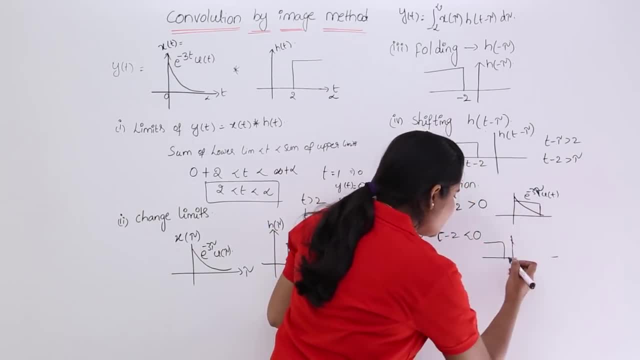 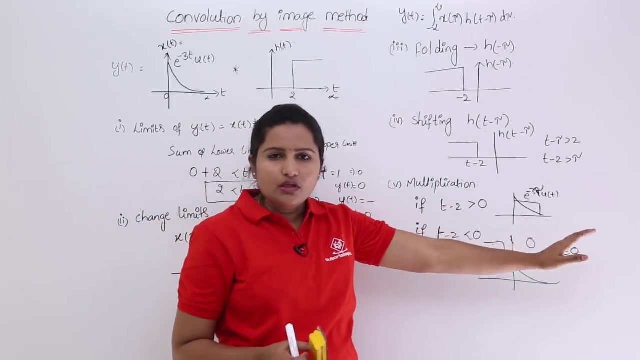 Why? Because Because you are going to multiply this signal with this signal- here this is undergoing this signal- into 0. here, this 0 into this signal. So totally you are going to get 0. So now, so to get any value, then the condition you need to consider is t minus 2 must be. 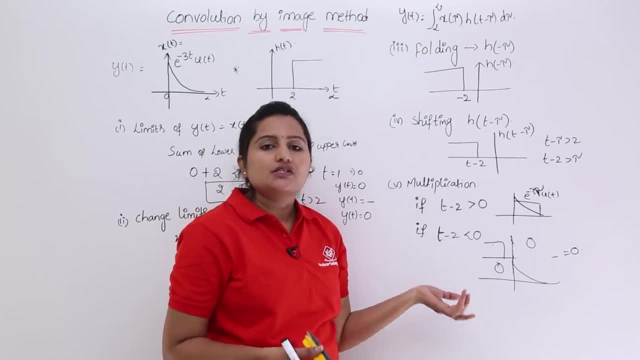 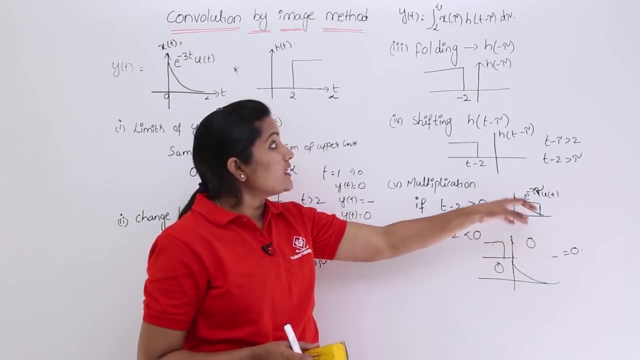 greater than 0. So otherwise you are going to get 0 as response of your convolution. So for this, how you will calculate means So definitely you will calculate, So definitely you can consider this integral integral. so this is so t minus 2 value. 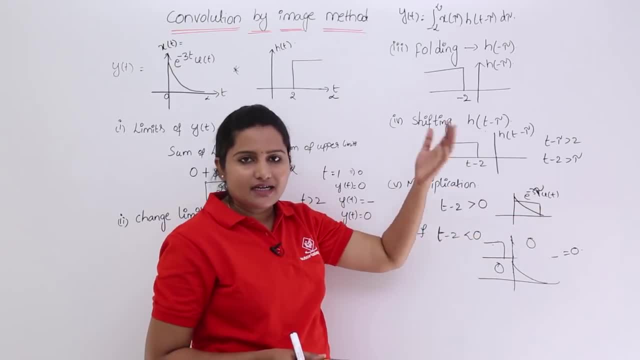 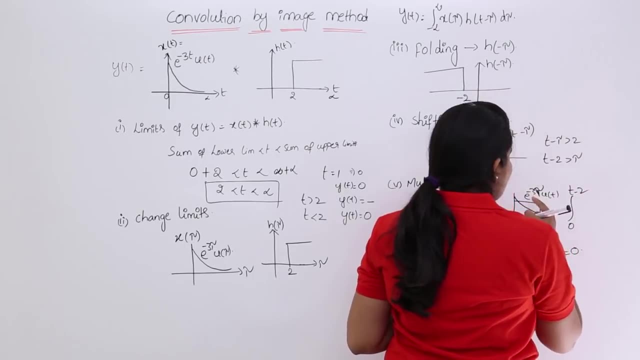 So this t minus 2 value you need to consider as greater than 2.. So 0 to t minus 2. so I am considering like this integral: 0 to t minus 2, multiplication of these two, 1 into e, power minus 3, tau into u, of t into 1.. 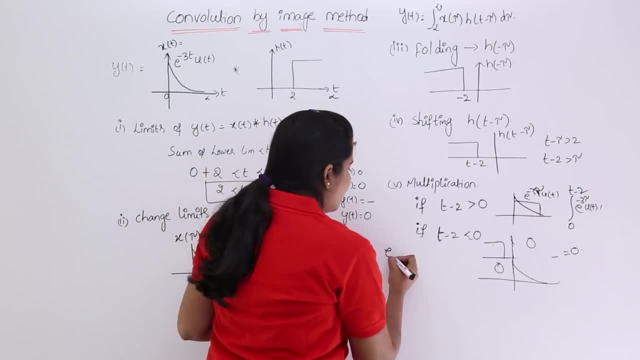 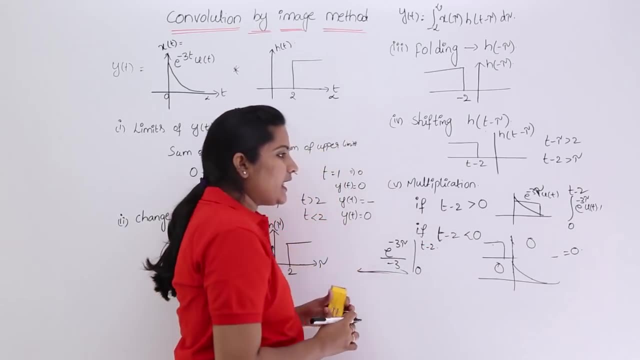 So here e power minus 3 tau means, So e power minus 3 tau by minus 3.. Ok, So e power minus 3 tau is equal to 0 to t minus 2.. So like this you can calculate that integral value. 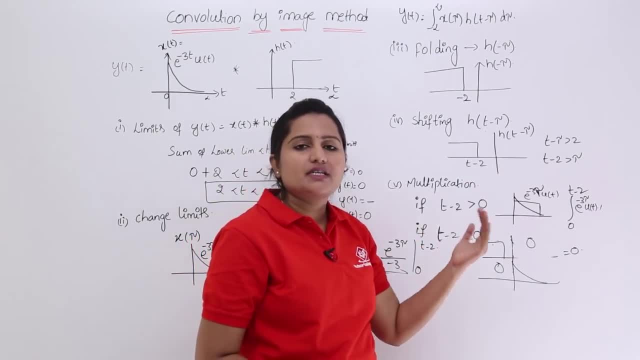 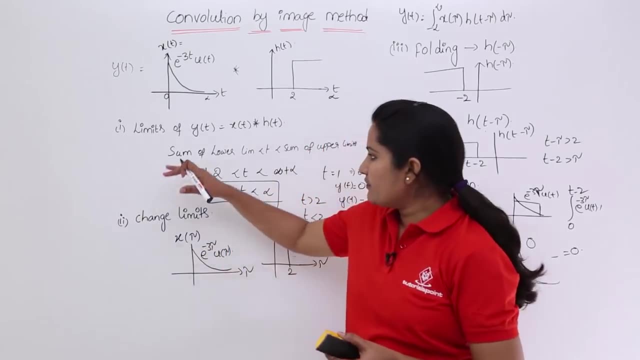 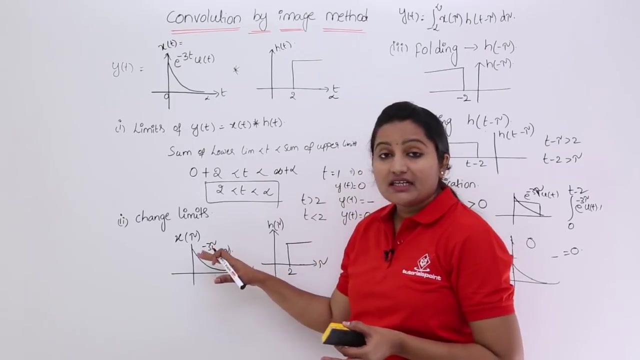 So here, after substituting this limits, you are going to get some value for this integration. So, whatever signals we given with for that, first we need to check the limits- that means lower limit and upper limit and lower limit- and after that you need to change your time.